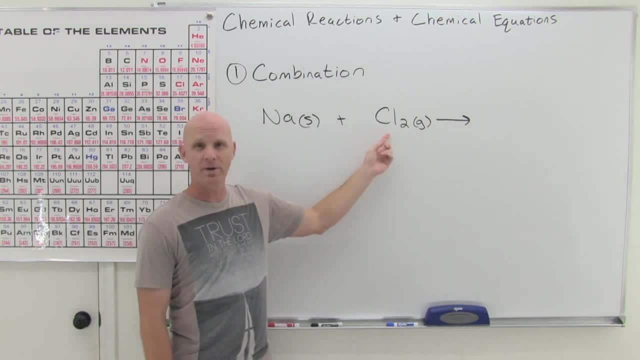 an elemental metal with an elemental nonmetal. You might recall from one of our early lessons that chlorine is a diatomic here, And when you mix a metal and a nonmetal in elemental forms, you're going to form an ionic compound, And so in this case we're going to form something that's a combination of sodium. 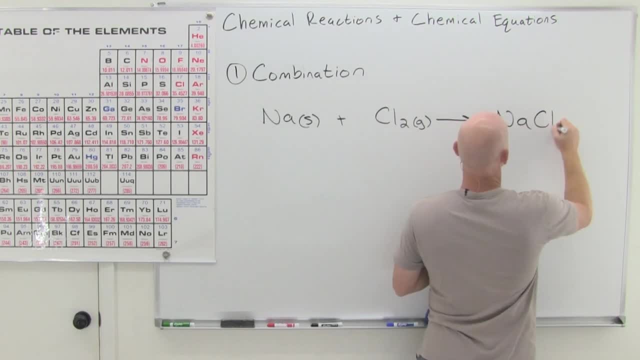 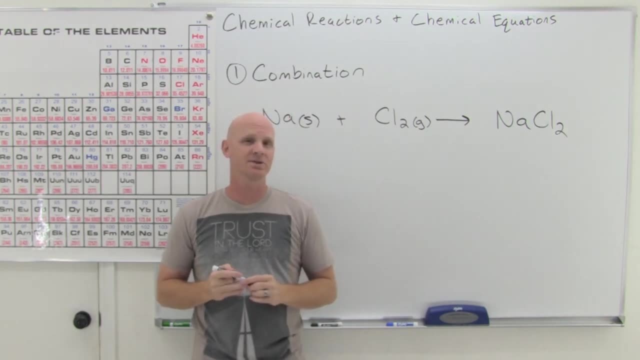 and chlorine. One of the big mistakes students make here is they just look at what they combined and, just you know, sandwich them together and go here. But what you might remember when we learned how to name ionic compounds in the last chapter is that a proper ionic compound has no overall charge. 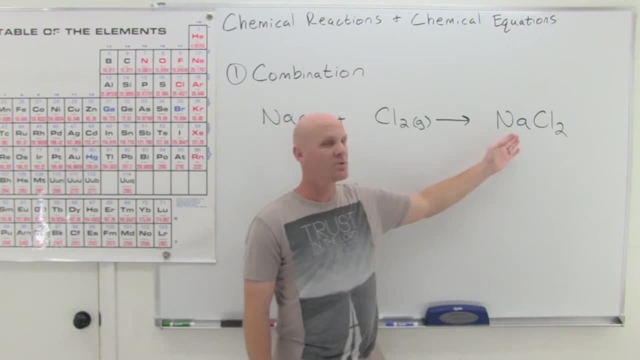 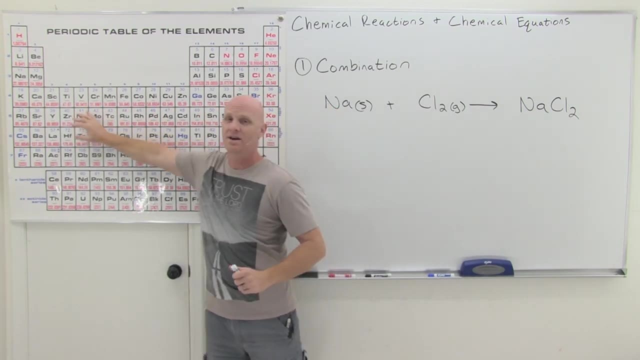 And unfortunately, that's this is wrong. We've done this incorrectly. So, if you recall, based on where monatomic ions are located on the periodic table, as long as they're not transition metals here or under the staircase, at least you can predict their charge. 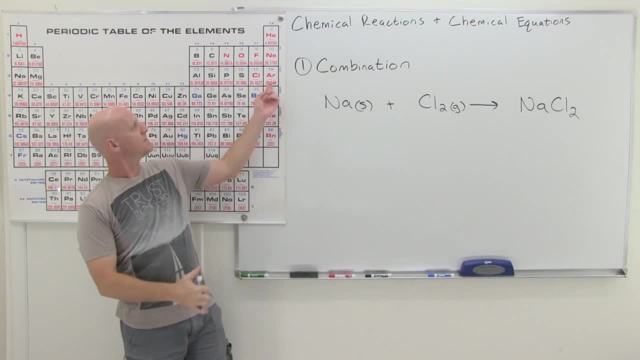 And so sodium is one electron beyond the previous noble gas, And so as an ion it's typically going to take a plus one charge. Chlorine is one electron short of looking like a noble gas, And so as an ion it's typically going to take on a minus one charge. 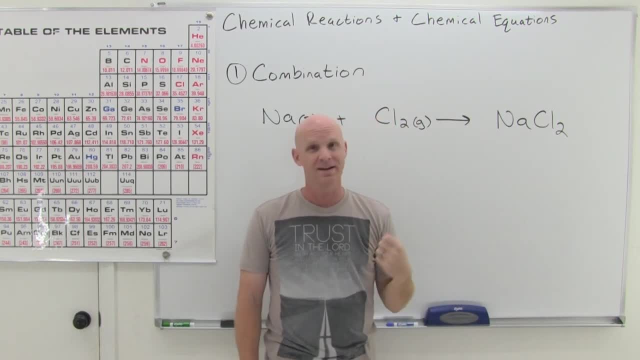 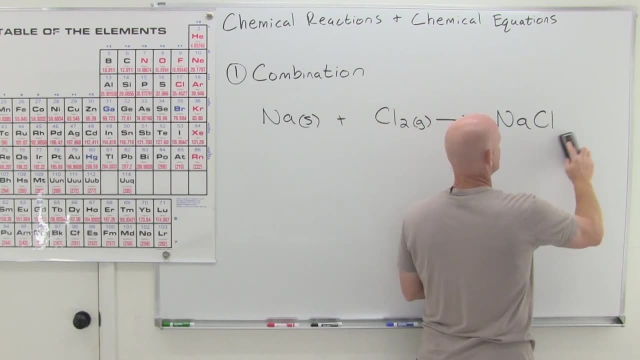 And so if sodium is plus one and chlorine is minus one, then we should only need one of each in the proper formula for sodium Chloride. And you probably already realize this was a one to one ratio, not a one to two ratio. 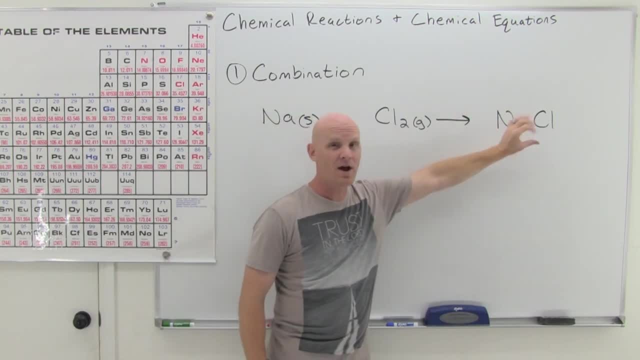 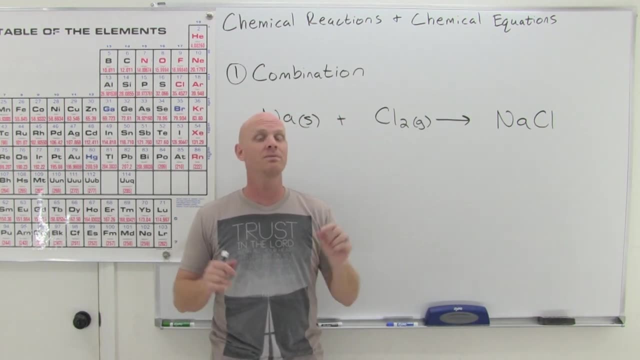 So that's the first thing. students often make the mistake, when they're predicting a product, of just carrying over some subscripts from the reactant side of the product side. But again, that's not necessarily the case When you form an ionic compound. 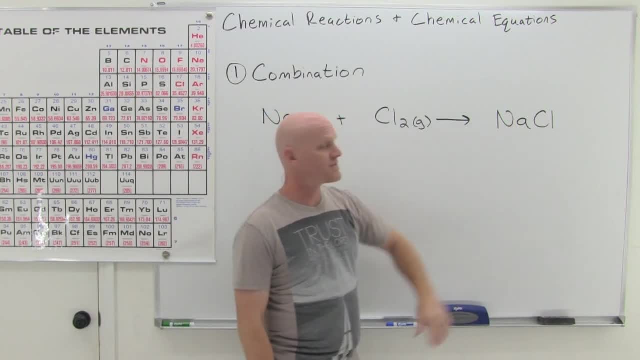 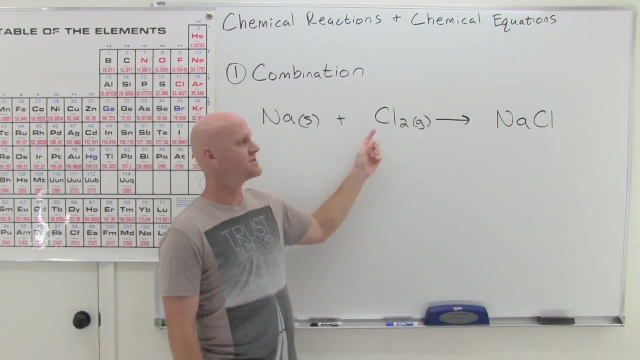 the key is, the charges have to balance out to zero. OK, so now we've got this part, Now we've got to balance this thing. And if we look here, the sodiums look good one to one, But the chlorines are not so good here. 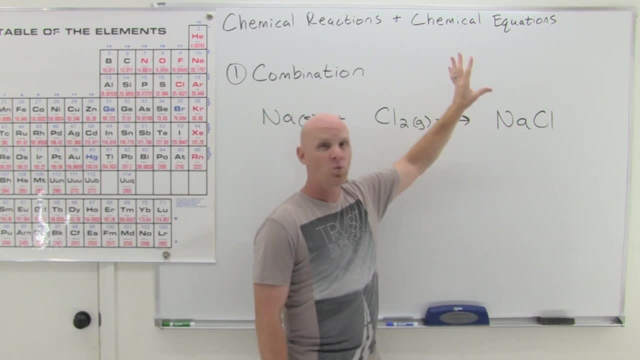 And so we've got two chlorine atoms on this side, only one on this side. And so once you get the proper formulas, you can't add any more subscripts over here, because that would again unbalance the charge. And so after you've got the correct formulas, 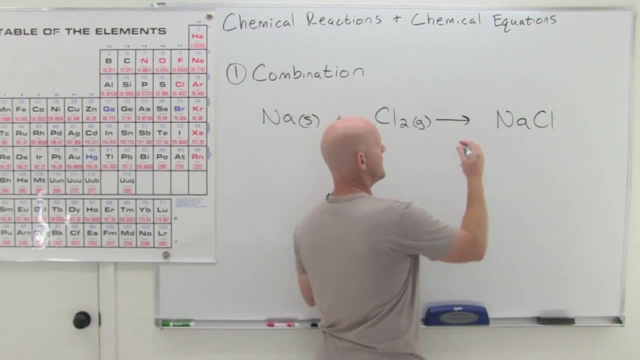 now you're going to put coefficients in front of chemical species, And so we're going to need to put a coefficient of two right in front of NaCl, and that's going to get us two Na's and two Cl's and that's going to balance out the chlorines. 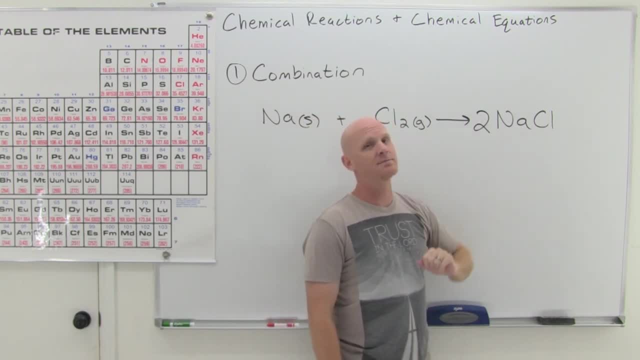 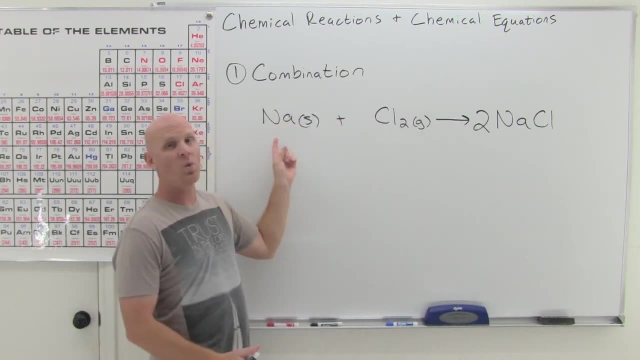 We've got two chlorine atoms on this side. We've got two chlorine atoms on this side, But even though the chlorines are now balanced, now the sodiums aren't, Because now we've got two sodium atoms on this side, We've only got one on this side. 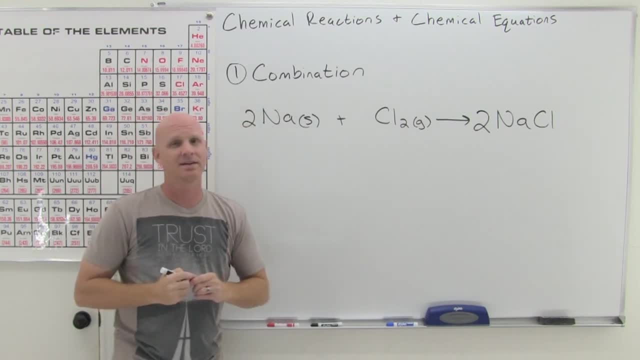 And so we're also going to have to put a two right here. And this is the balanced combination reaction. And again, you can recognize this as a combination reaction because you've got two reactants and only one product, And so that's the hallmark of a combination reaction. 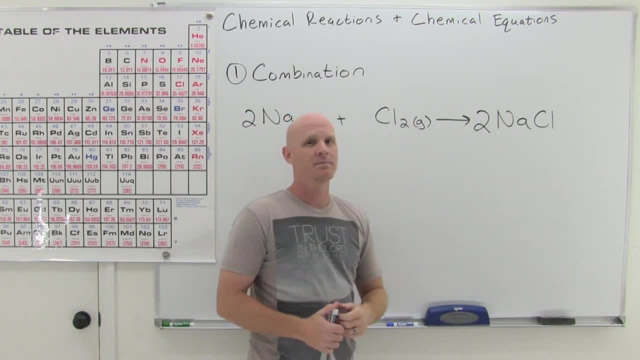 You've got two or more reactants forming just a single product. Now the second type of reaction we're going to look at is the exact opposite of this, As far as how you recognize, and it's called a decomposition reaction. And in a decomposition reaction, 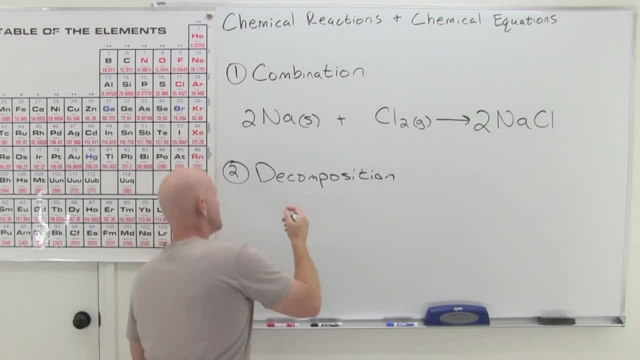 you're typically going to have a single reactant breaking up into multiple parts here. So the one I've got on the study guide here has calcium carbonate, So in this one we don't expect you to be able to predict products usually, So I'm just going to give you the products on this one. 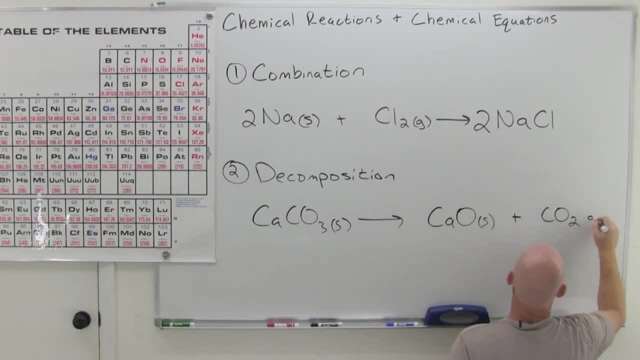 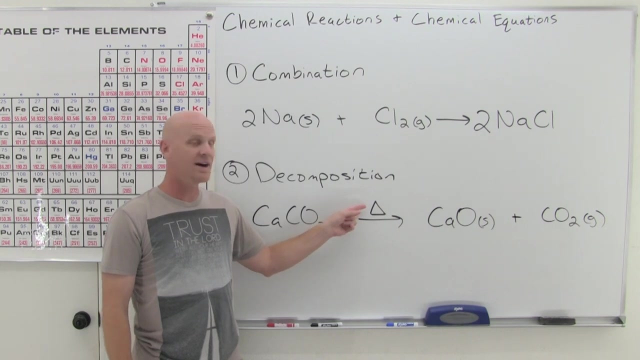 So we're going to form some calcium oxide and some carbon dioxide gas, And it turns out most of these decompositions are what we call a thermal decomposition, which means they require heat. And one thing you'll find out along the way is that oftentimes we use this lovely triangle, which is the Greek letter delta. 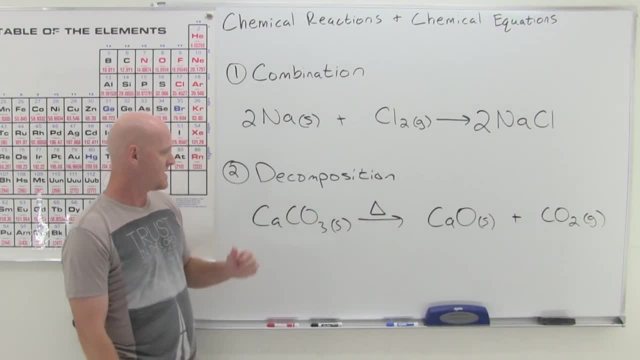 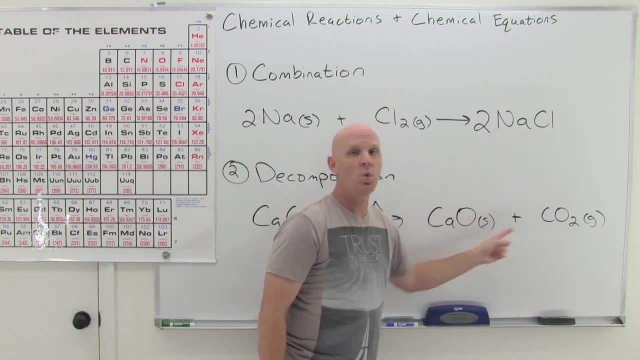 to represent heat, And so this means the application of heat here, And in this case this is a decomposition. first, And you can recognize it, because we only have one reactant, but we have more than one product, So that's decomposition. 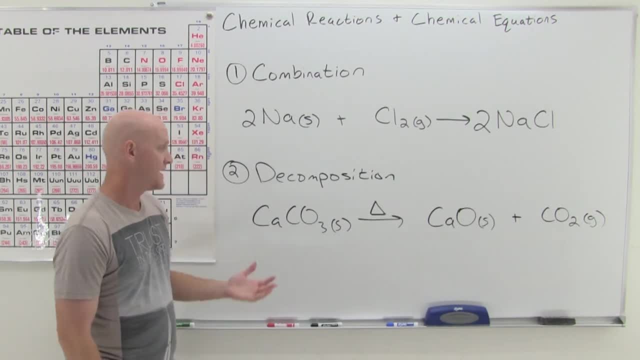 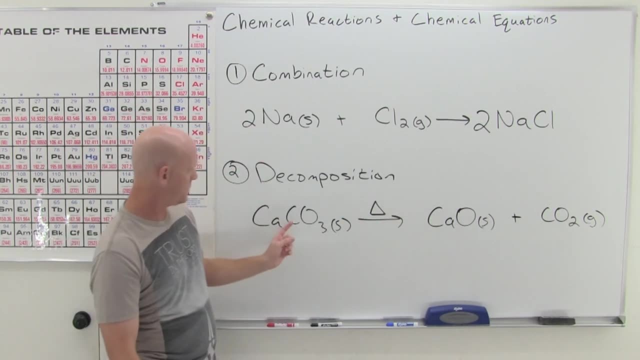 Whether the heat's written in there or not, it would still be a decomposition reaction, And if we look, though, what's nice is that this is completely balanced. in this case, We've got one calcium, one calcium, one carbon, one carbon, three oxygens. 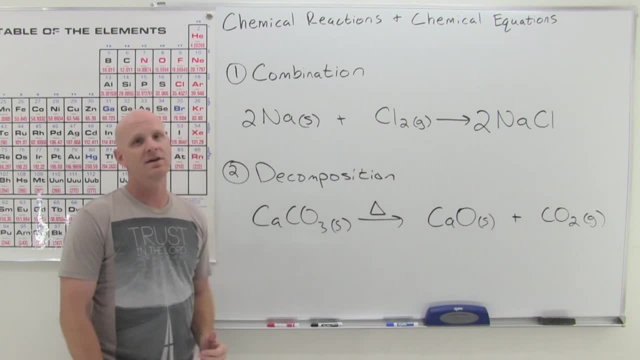 One, two, three oxygens. It's completely balanced. Don't have to add any coefficients. Now, one thing to note- and I probably should have said it right up here- is that when you don't put a coefficient in front of a reactant, 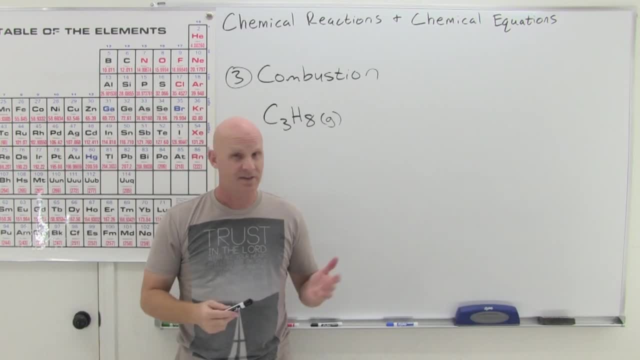 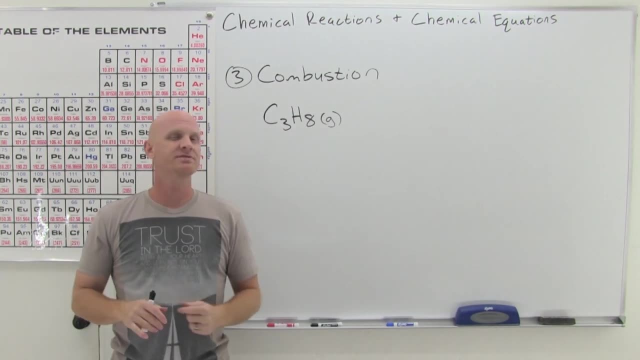 it's automatically implied that there is a one there. All right. The next type of reaction we're looking at is called combustion, And one you're probably somewhat familiar with. It's like like burning something, And the question I might ask you is: why can't you combust something on the moon? 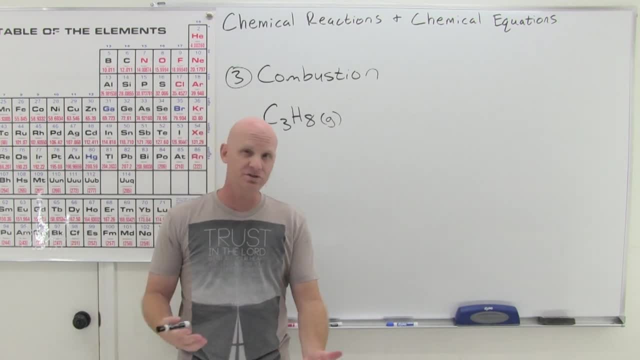 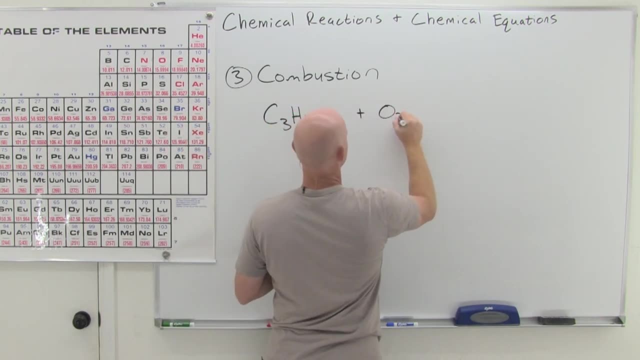 And the key is is there's no atmosphere on the moon And so there's no oxygen on the moon. And so it turns out that combustion, simply put, is the reaction of something with oxygen, gas. And so you know how do you put out a fire. 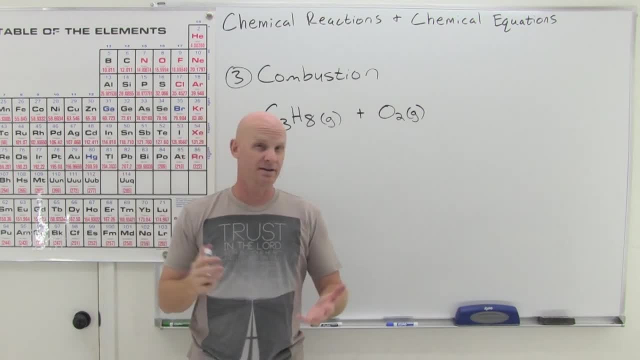 Well, you could cover it in water, So. but I don't know if you've ever seen like a fire blanket. A lot of chemistry labs are equipped with a fire blanket And if somebody catches fire you can wrap them in a blanket. 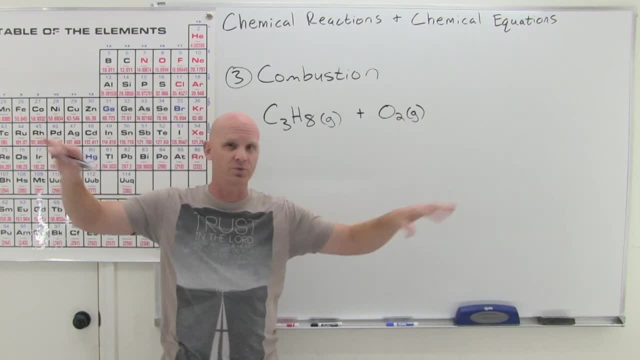 And what you're really trying to do is separate them from the oxygen in the room. If you limit the oxygen that the fire has access to, you can limit the fire and potentially even put it out. Same thing you might have seen, you know, burning something flammable in a beaker. 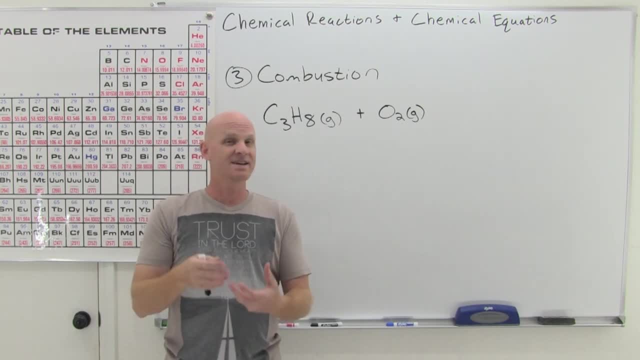 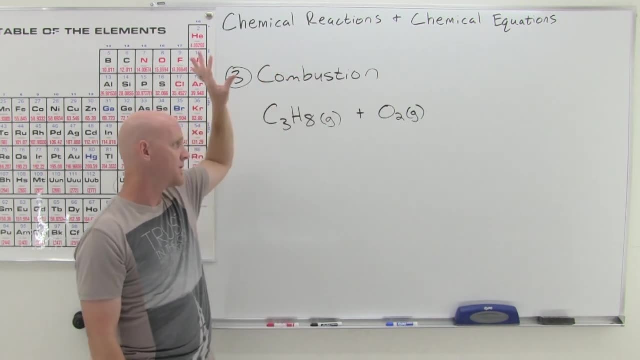 If you put a watch glass on top, once the oxygen that's inside that beaker is all burned up, the fire goes out. So you need oxygen to have a fire. So you need oxygen to have combustion. So combustion of something is always going to be a reaction of it with oxygen. 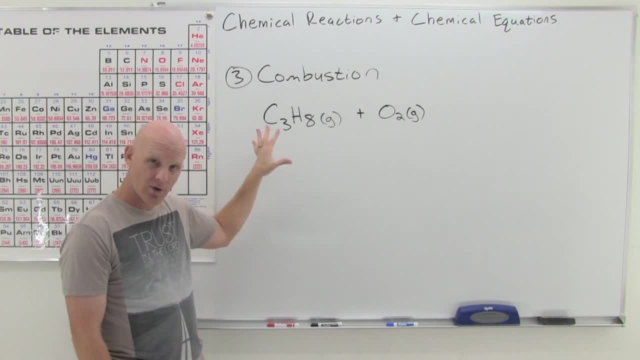 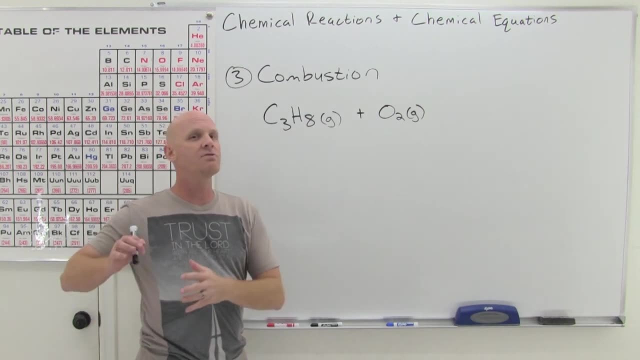 In this case, we'll look at the combustion of this is turns out propane- Don't expect you to know that at this point- but really the combustion of propane and technically you can do combustion of things other than hydrocarbons. But we are specifically in this lesson, going to look not just at combustion. 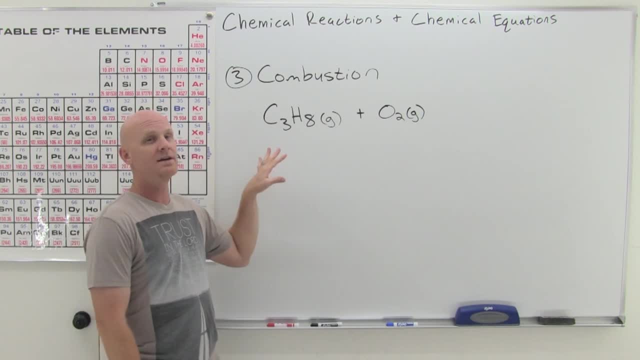 in general. but the combustion of a hydrocarbon, and a hydrocarbon is an element made of just hydrogen and carbon. Now, technically I could still put a hydrocarbon that also has oxygen in it, which technically makes it more than a hydrocarbon at that point. 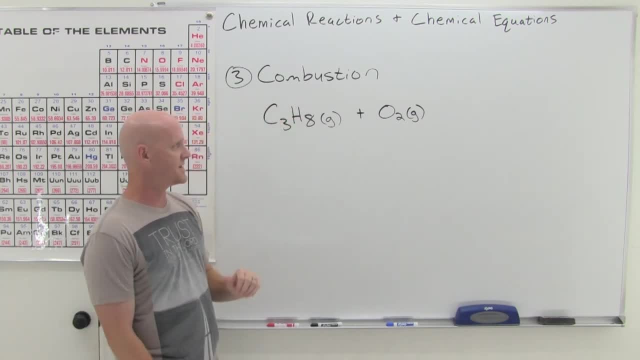 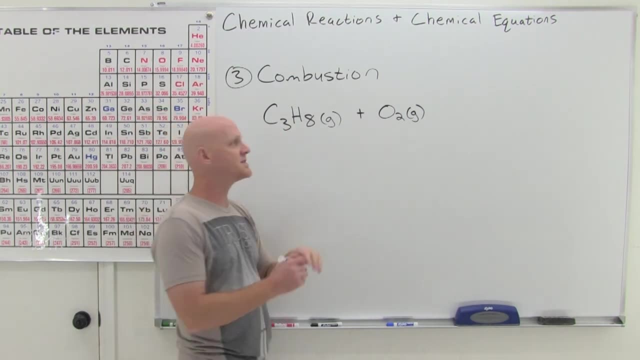 And that's fair game. But no other elements are we going to involve at this stage of the game. So combustion of a hydrocarbon: So you have a hydrocarbon variability here in what that exact hydrocarbon is, but plus oxygen and for a hydrocarbon when you do combustion. 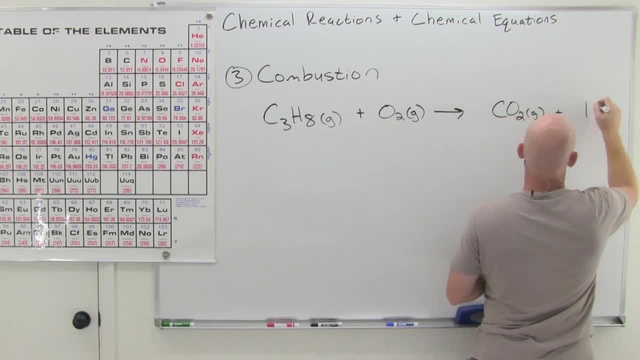 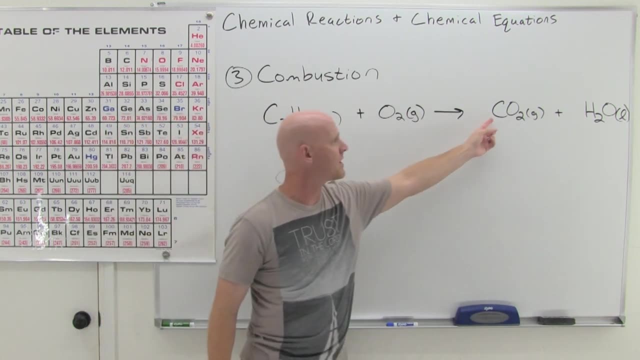 you're always going to form carbon dioxide and water. So it turns out all the carbons from that hydrocarbon are going to end up as carbon dioxide and all of the hydrogens in that hydrocarbon are going to end up as part of water. 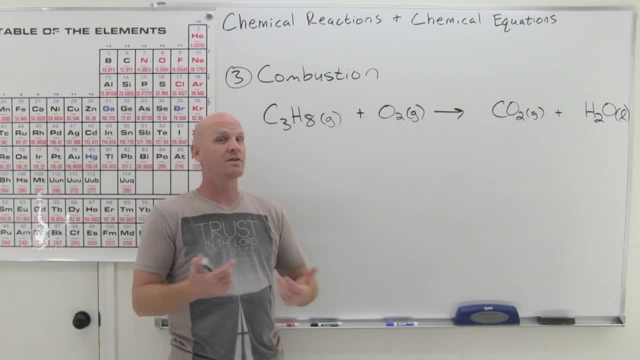 And we expect you to be able to do that. You're going to be able to predict those products and even know what the kind of the combustion reaction looks like. Now, when we go to balance this- though, this is one of those reactions that's one of the more difficult ones to balance- 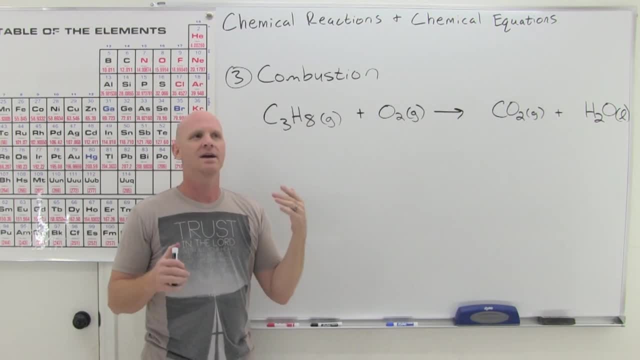 And sometimes you go to balance one like this and it just works out And you're like, OK, that was easy. And then sometimes you go to balance it and you just go back and forth and you can never get the thing quite balanced. 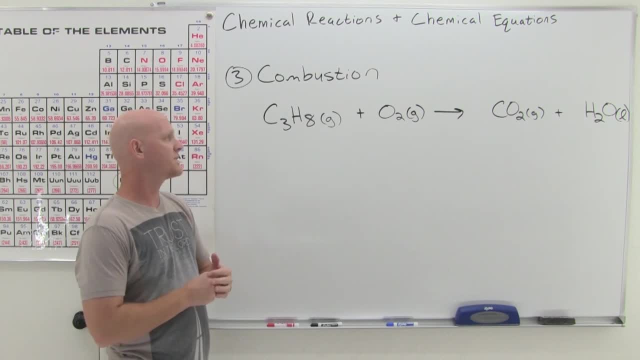 And so we're going to kind of take the mystery out of that and see why that works out that way. So it turns out this is a good example of one of those pesky balancing ones And what you want to look for when you're. 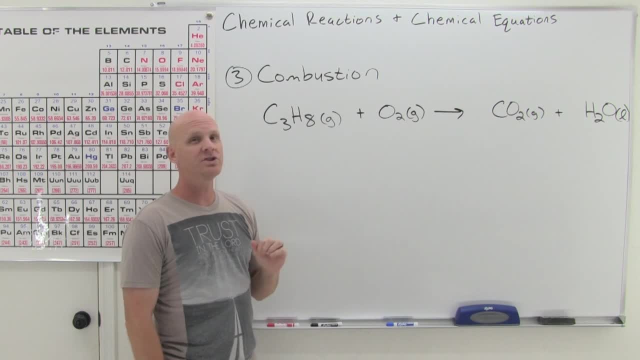 balancing a reaction is specifically an element that only shows up in one location, on both sides of the arrow, in either one element or one compound. Well, we have an element here and then the rest of these are compounds. But if we look at, say, carbon for instance, carbon only shows up in this. 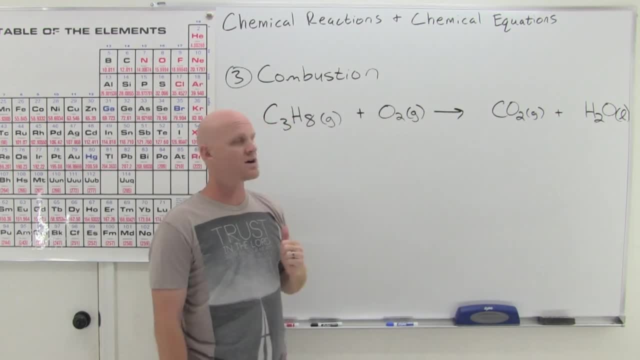 one reactant and in this one product. that would be a good place to start. If we look at hydrogen, hydrogen only shows up in this one reactant and this one product. that would be a good place to start. Oxygen shows up in this one reactant, but it. 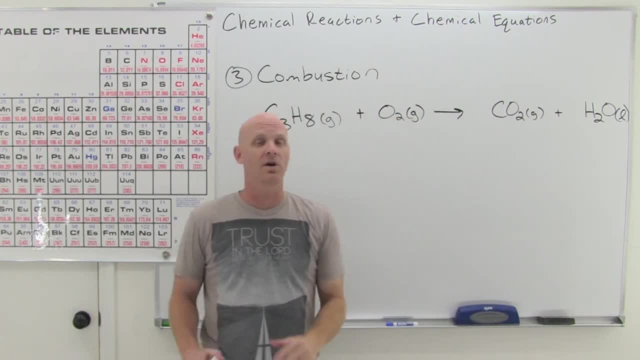 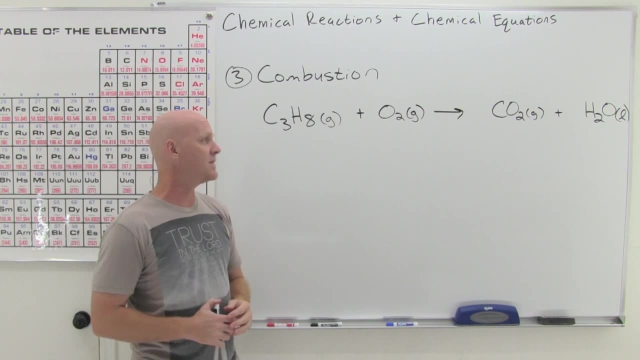 shows up in more than one product. That would be the worst place to start, And if you start with oxygen, that's when you're going to run into problems. But as long as we start with carbon or hydrogen, no problems in balancing this thing. 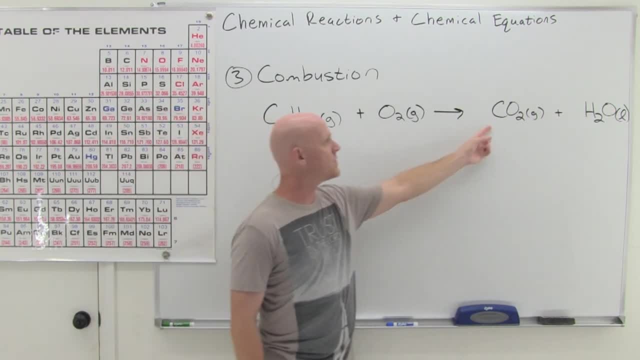 So let's start with the carbons. So here we've got three carbons, Here we've only got one. We've already got all the proper formulas, So we can't change any subscripts from here. We can only put coefficients in. 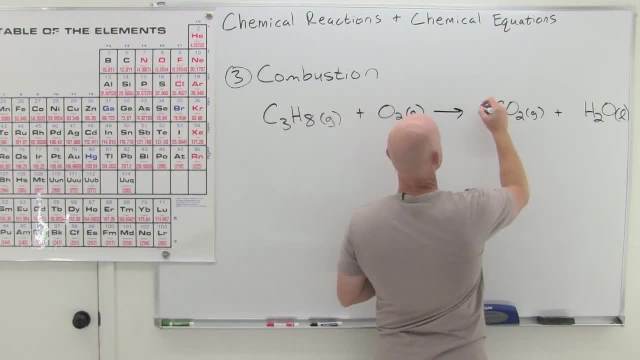 And so to get it so that I've got three carbons on this side as well, I've got to put a three right here. So, and once again, we don't want to balance oxygen yet, We want to Save that for the end. 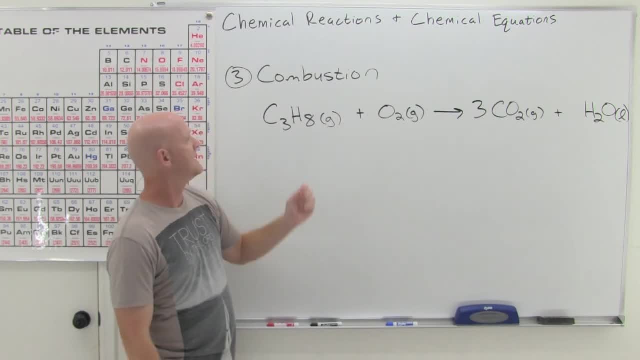 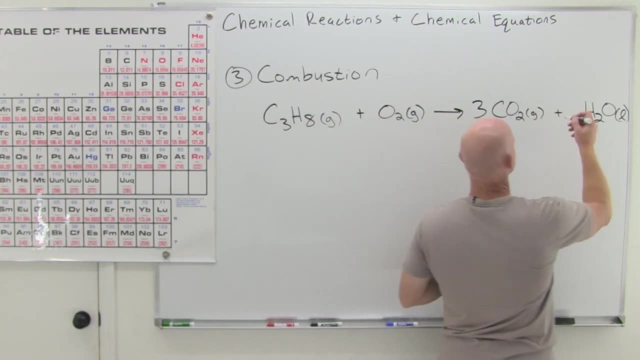 So we'll do hydrogen next, since he only shows up in one reactant, one product, And we've got eight hydrogens on this side. We've only got two on this side, So to get a total of eight on this side as well, we're going to need to put a coefficient of four in there. 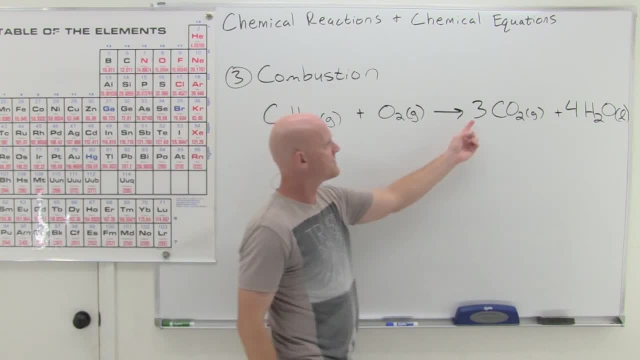 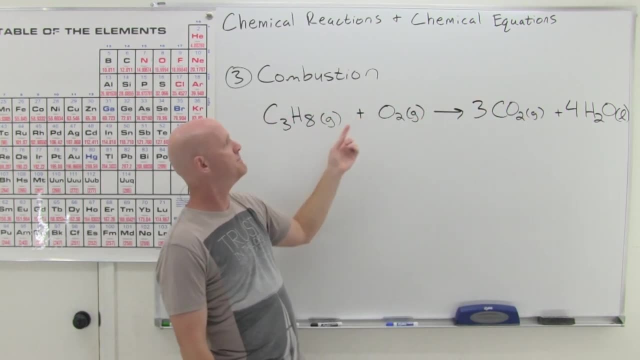 And what's nice is now we're at a point where we can deal with those oxygens because we've already set the coefficients for these two, so that also sets the total number of oxygens is fixed, and then we can balance it by putting a coefficient over here. 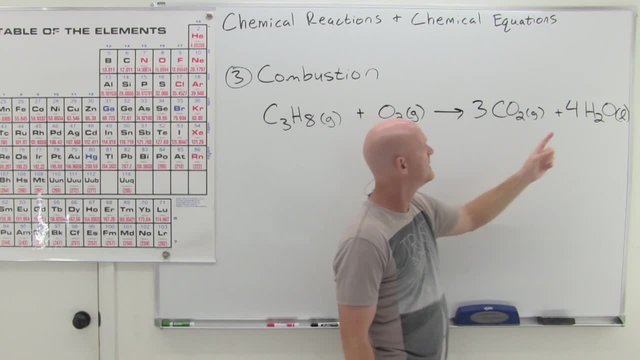 So in this case two, we have six oxygen atoms here. Four times one is another four oxygen atoms, for a grand total of ten oxygen atoms. To get a total of ten on this side, we're going to need five O2s. 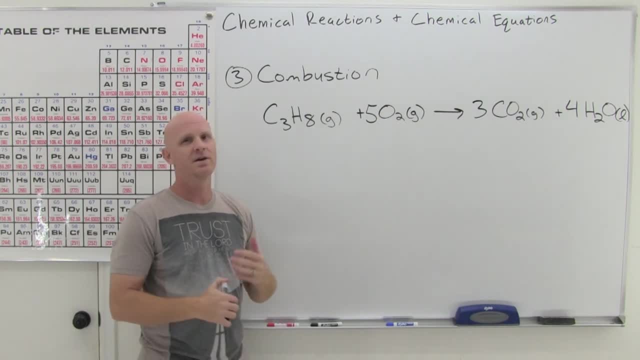 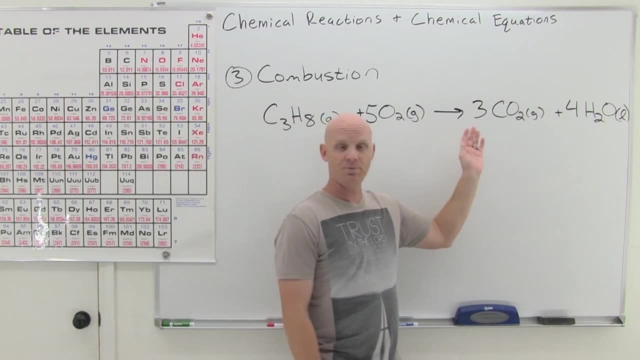 And this is the balanced reaction for the combustion of propane. And again you should recognize it as combustion of a hydrocarbon, because again it's hydrocarbon plus O2.. And again your products are going to be CO2 and water every time. 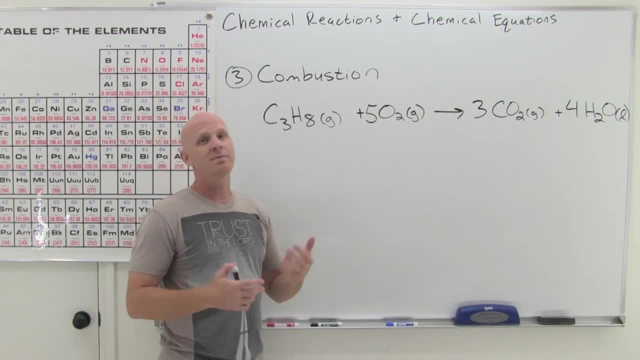 at least in the context. you guys see it Cool. So that's combustion. You might expect you to be able to predict the products, or even predict everything but the hydrocarbon. After the hydrocarbon, these three other species are all fixed. Oxygen is always the other reactant. 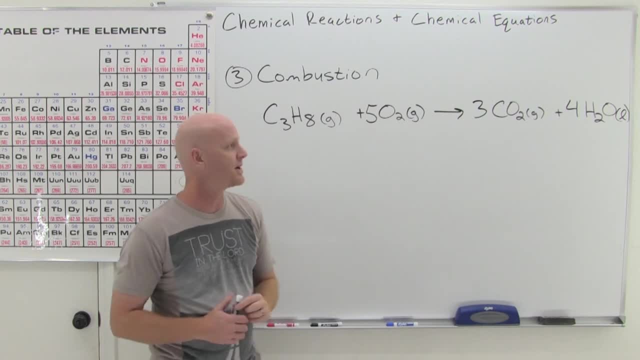 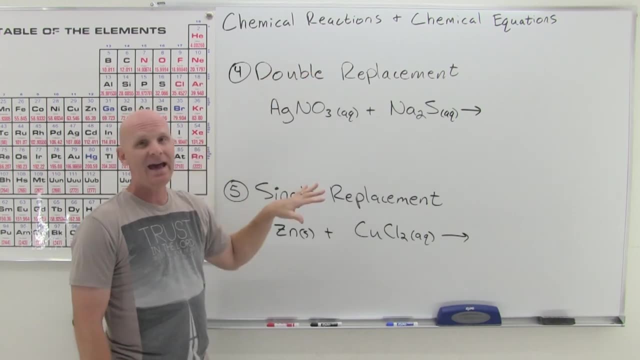 and CO2 and water are always the products in the combustion of a hydrocarbon. All right, The last two kind of reactions we're going to look at are somewhat similar, So I want to cover them together here. And we've got double replacement and single replacement. 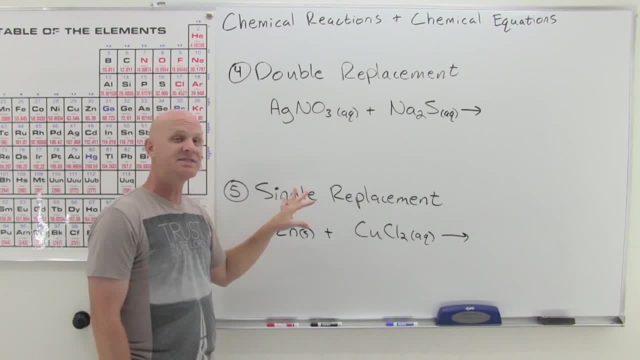 Now turns out these can also be called double displacement and single displacement, So you might see it there as well, And we're actually going to see these both again in chapter four, And we'll actually learn that double replacement reactions also go by the. 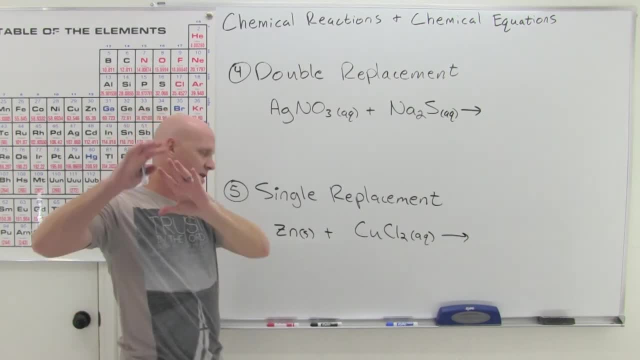 names like metathesis and exchange reactions, And we'll cover that in much more detail in chapter four. But at this point I just want you to be able to recognize these kind of reactions and stuff. And it turns out both these are examples of what we call aqueous reactions. 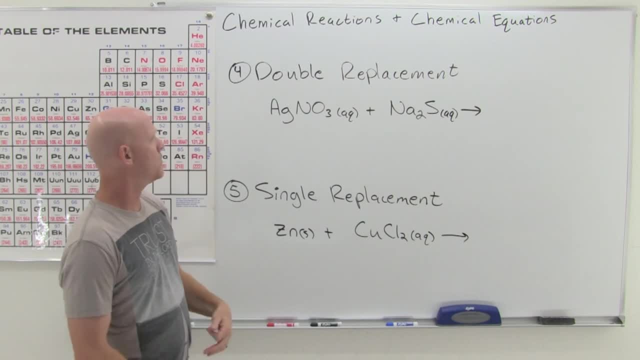 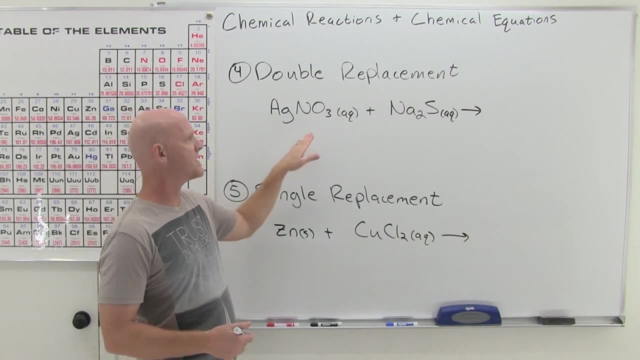 They typically take place in water as a solvent, So they're dissolved in water, And in this case, we want you to be able to predict products for both of these, as well as be able to balance, And so in this case, it turns out in a double replacement reaction. 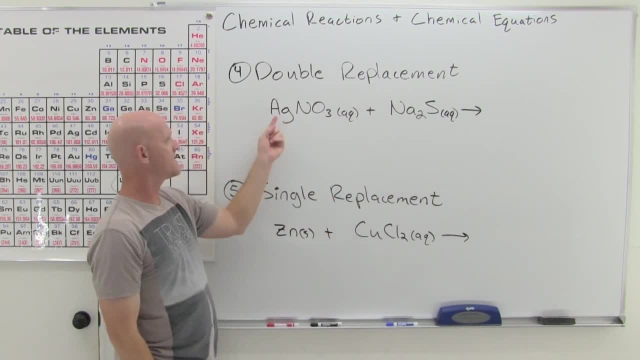 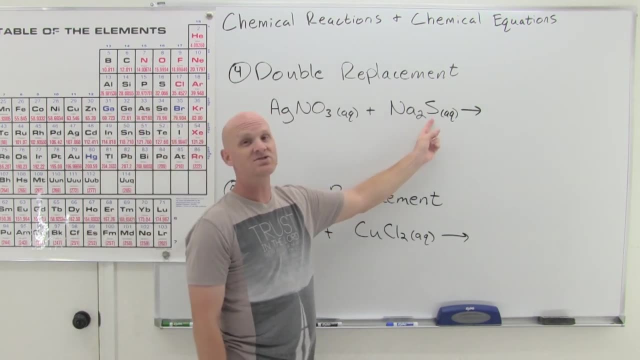 you're just going to have cations and anions, trading partners. So here we've got cation, Here's the silver ion, The anion is the nitrate polyatomic ion. Here the cation is sodium ion and the anion is the sulfide ion. 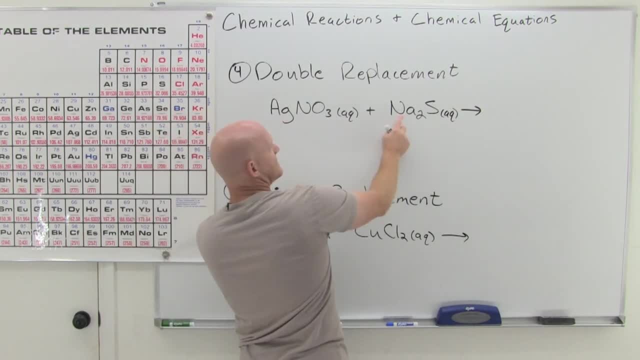 And we're just going to trade cations and anions- This cation is going to go with this anion and this cation is going to go with this anion- And we'll just rewrite those products. And so in this case, we're going to have silver. 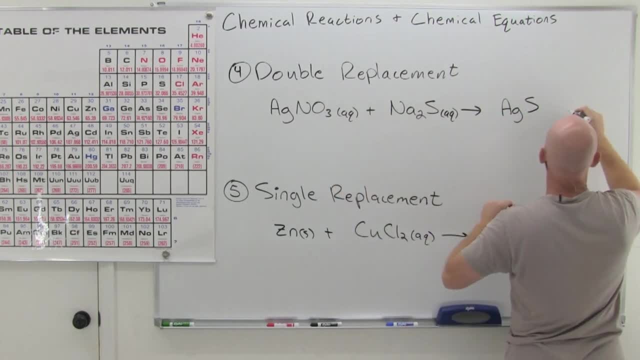 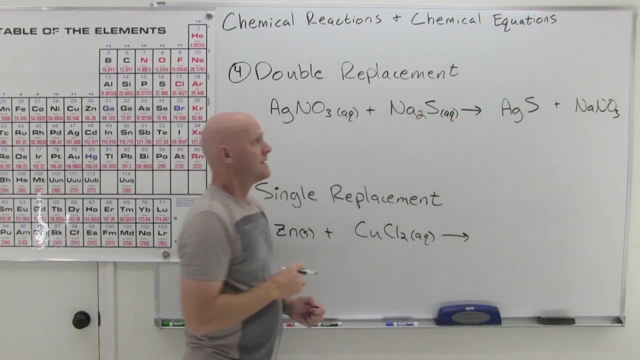 going with sulfur and then sodium with nitrate, And we always write the cation before the anions: Sodium first, nitrate second. All right, Now we've got to get these formulas correct And once again we've formed ionic compounds here. 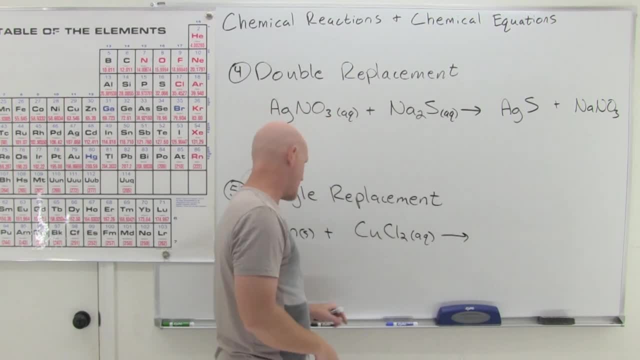 And the proper formula for an ionic compound has the charge balanced out to zero, And so in this case, if you've memorized that you know that nitrate is minus one, then you could figure out that silver here is plus one. 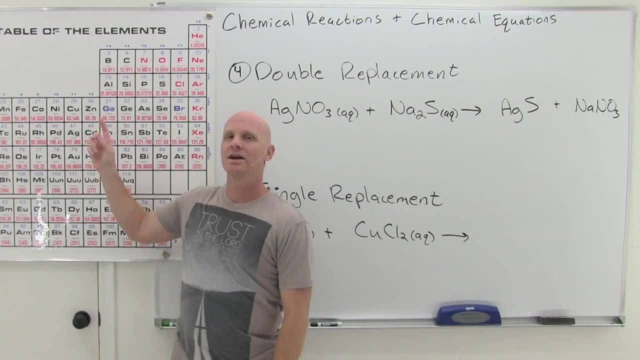 But silver, even though he is a transition metal, he was one of those four that always gets the same charge. Silver as an ion is always plus one, Zinc and cadmium are always plus two and aluminum was always plus three. So, even if you didn't know, the nitrate was minus one. 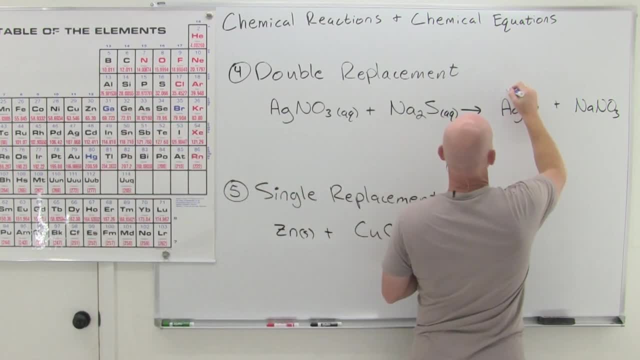 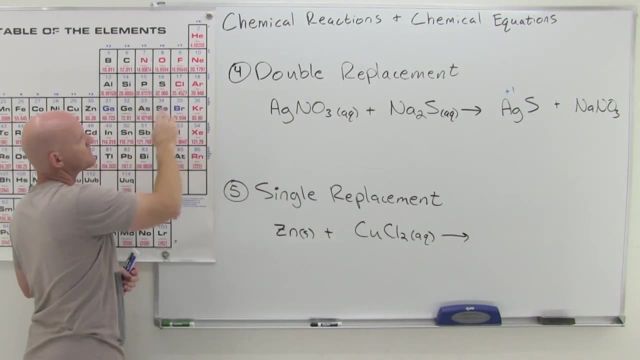 silver as an ion is supposed to be plus one anyways. And so here he is as plus one, And in contrast to that we've got sulfur right here, And sulfur as a monatomic ion wants to gain two electrons, we like to say, and look like argon. 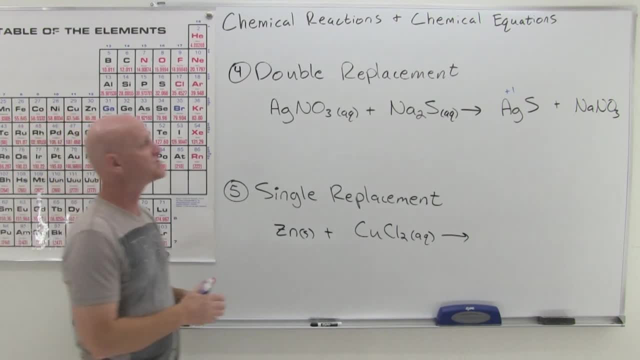 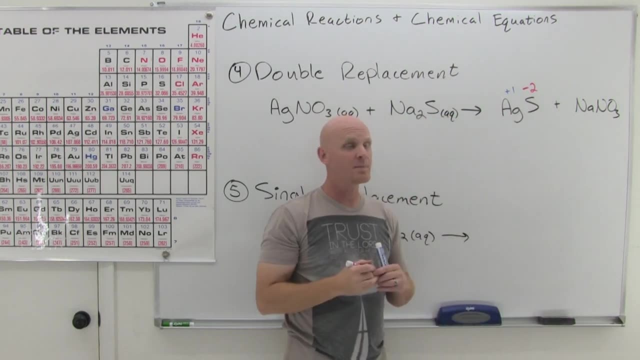 So in gaining two electrons to look like a noble gas, he would have a minus two charge as a monatomic ion here, And so we can see that the charges are not balanced, And so that is not the proper formula here. So we have more minus than we do plus. 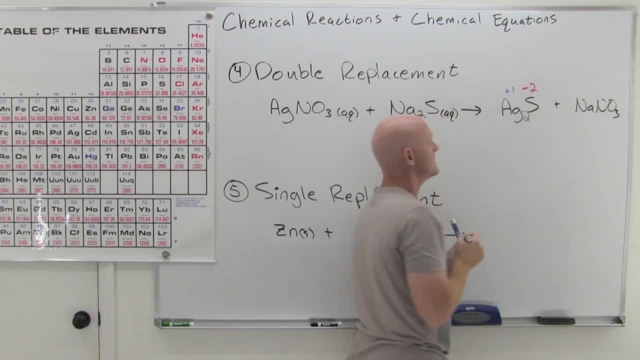 And so we're going to have to put a subscript here in the formula so that I have two silver ions for every sulfur, and that way I've got a total of plus two to match up with that total of minus two, And this thing is now a proper formula here. 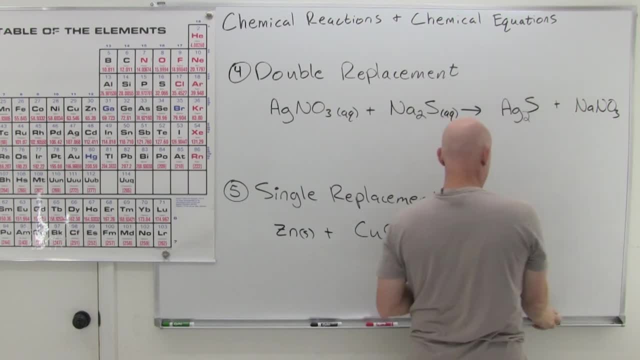 So these have served their purpose. We've now got the proper formula for silver sulfide and for sodium nitrate. So it turns out that your nitrate ions again, or your sodiums are plus one And your nitrate It's a polyatomic ion. 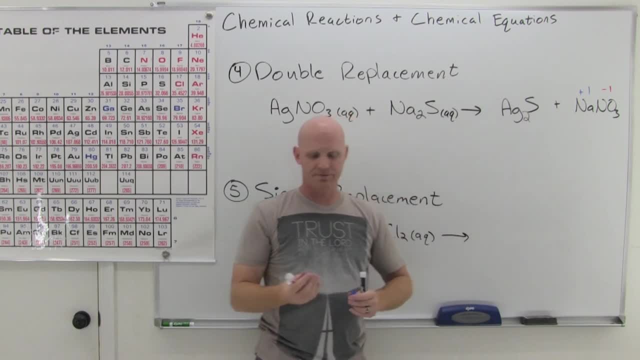 You're supposed to memorize that as minus one. And that is already the proper formula for sodium nitrate, balanced right out of the chute here, All right. So now that we've got the proper formulas, now we've got to go make sure it's balanced and adjust coefficients as needed. 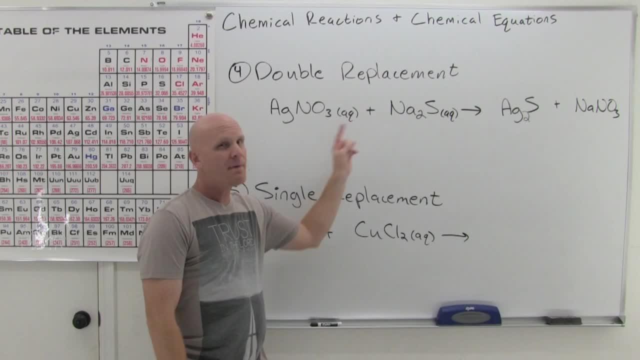 So what's nice about a double replacement is usually you can ping pong back and forth, So like, if we look at silver, one silver, Well here we've got two, And so we're going to need to put a coefficient of two right in front of here. 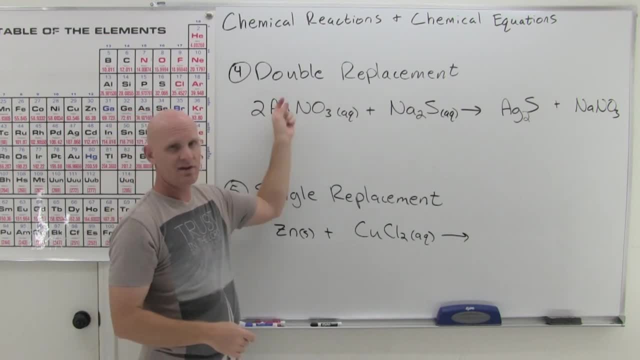 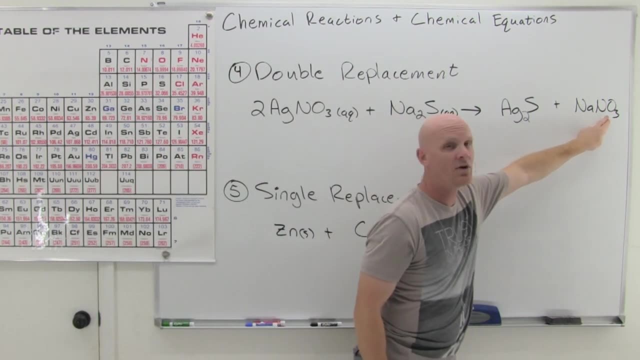 So if you put two silvers here, that also means you're going to have two nitrates. And what's nice about a double replacement reaction is it turns out So, because your polyatomic ions are going to stay the same polyatomic ion on both sides, it turns out you don't actually. 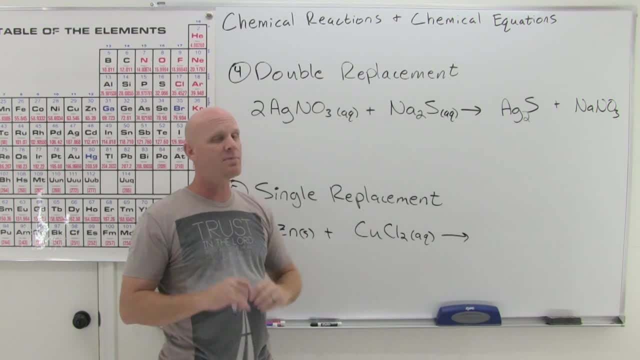 have to balance the nitrate and the oxygen separately. You can just balance the nitrate polyatomic ions, and it'll make sure that those nitrates and oxygen get balanced, And so in this case we've got two of these NO3s. 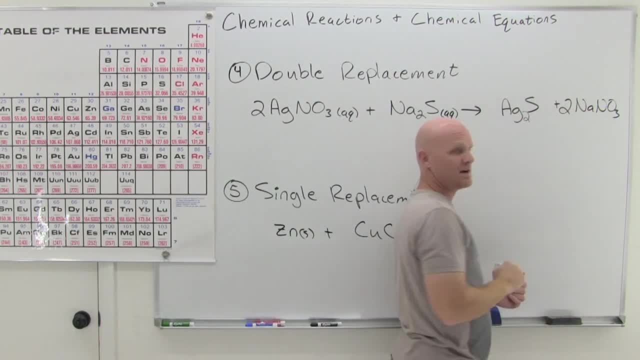 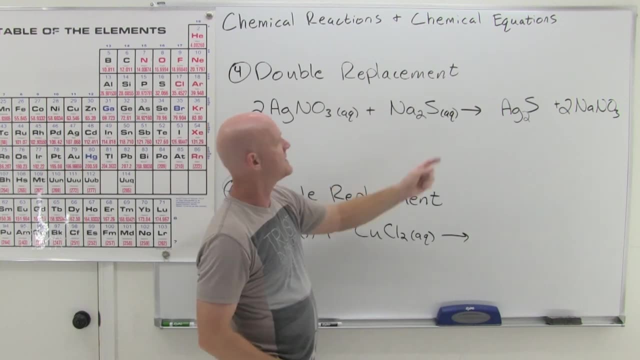 Here we've only got one, So I'm going to need to put a coefficient of two here. But that two not only gives me two nitrates, but it gives me two sodiums, and I've got two sodiums and then one sulfur, one sulfur. 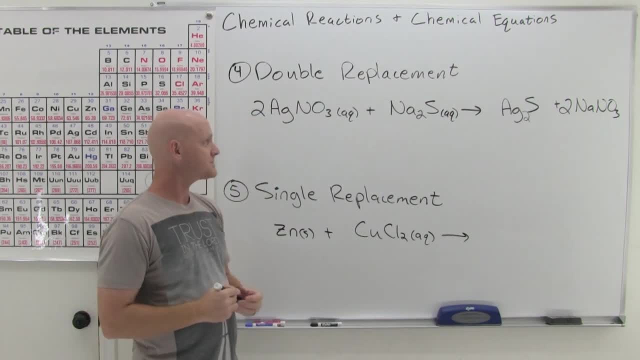 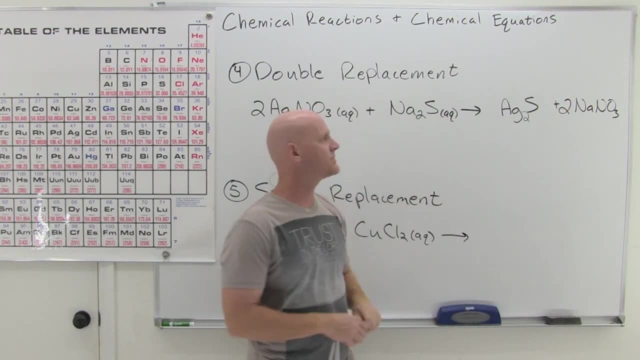 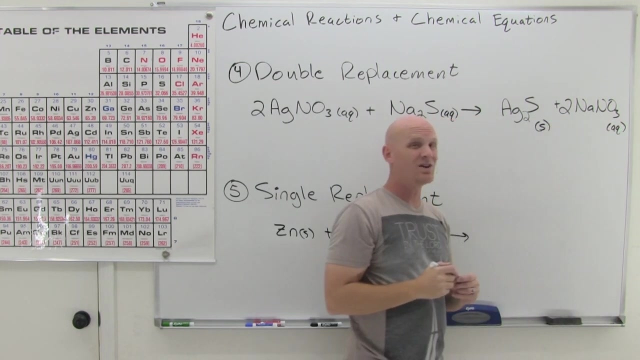 And this is now a balanced reaction. Now one thing to note. if you notice, I haven't actually put phases over here, and we'll learn in Chapter four how we actually do that. So, but it turns out that sodium nitrate would be aqueous and silver sulfide, though it turns out, is not soluble. 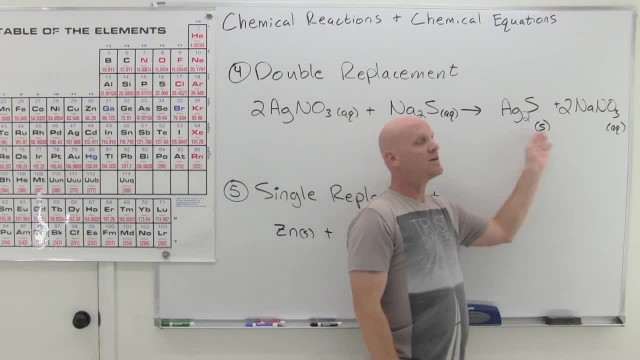 in water and would actually form a solid in the solution. And I don't expect you to be able to predict that now. But what we're going to give you in Chapter four we're going to be called solubility rules and the rules. 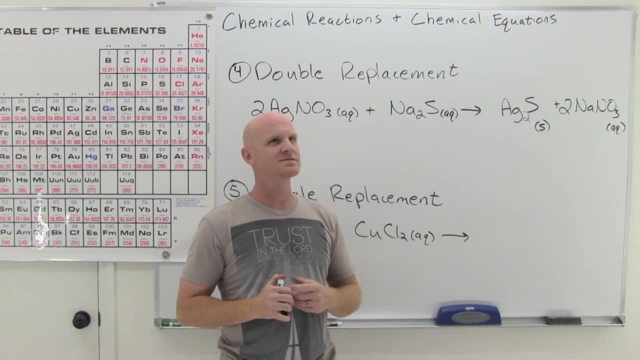 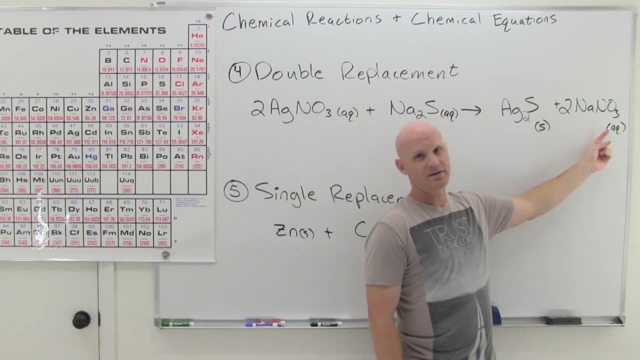 that you can, most of the time, look up every once in a while. A professor makes students memorize them, but they will allow you to predict whether or not something is soluble, And when it's soluble- we say it's aqueous- It'll be exist as dissolved in the water. 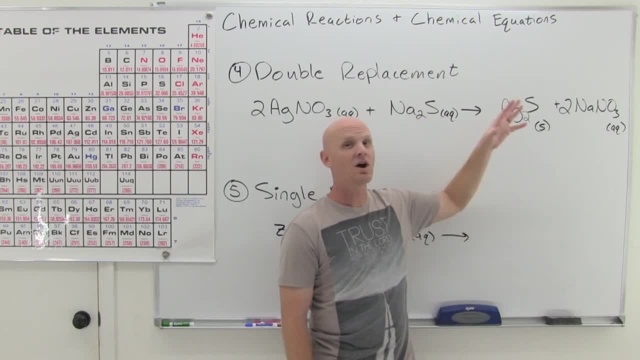 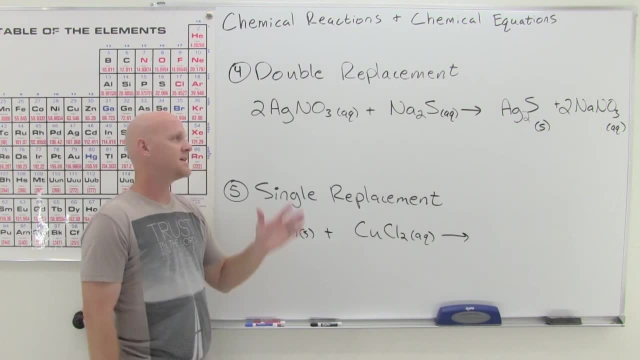 But when it's insoluble, it will not be dissolved, And so it'll be a solid that will usually settle on the bottom of your beaker, or what have you Cool. So those are double replacement reactions, And now we've learned how to predict the products and balance them. 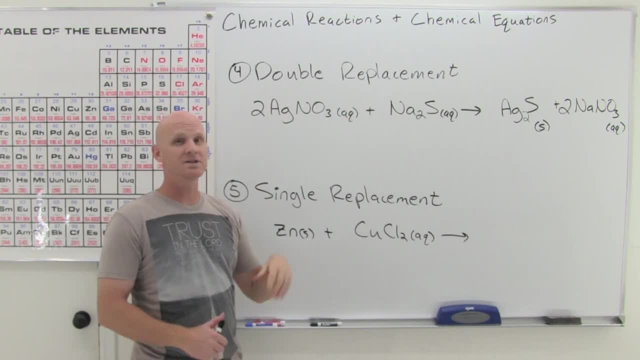 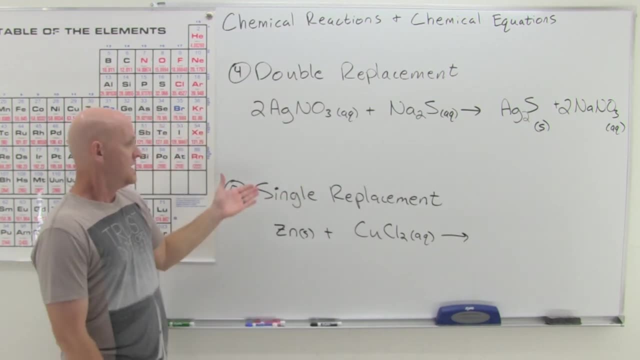 We'll find out in Chapter four that there are really three major types of these double replacement. So we'll even learn that within this one type of reaction there's multiple subtypes, if you will. So single replacement reactions: these are often reactions that take place in water as well. 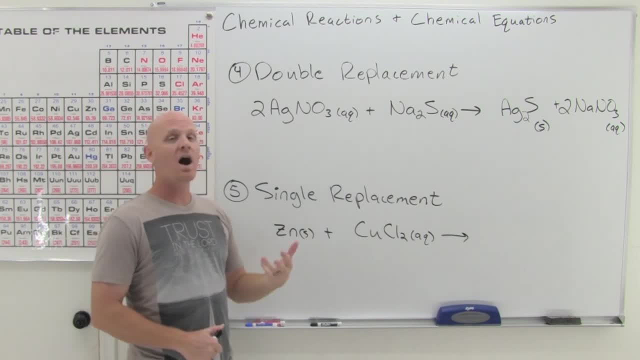 So in this case they're also what we call a type of oxidation reduction reaction, or a redox reaction for short, And so we're covering five types of reactions in this chapter. It's not an exhaustive list. There are other types and they're also different ways of classifying. 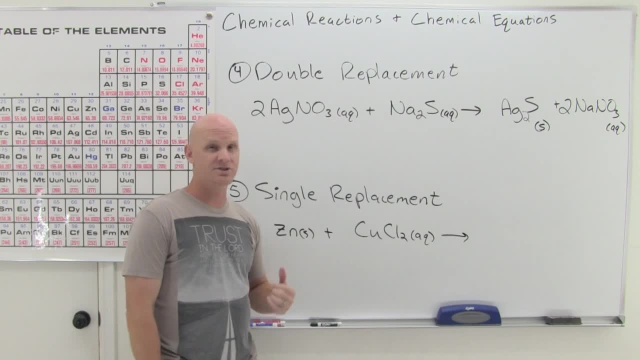 reactions, And so it turns out that this is an example of what we call an oxidation reduction reaction, but it also turns out that so was combustion, And we're not going to cover oxidation reduction reactions in this particular lesson, or even in this chapter. 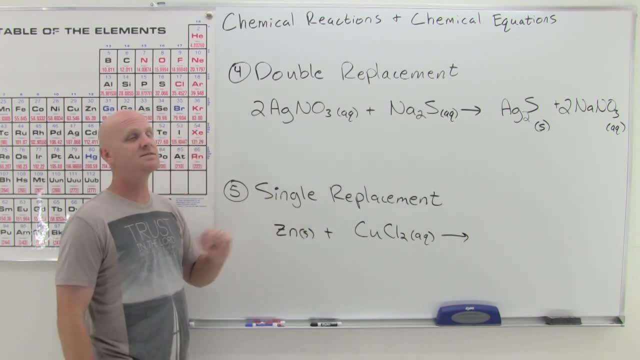 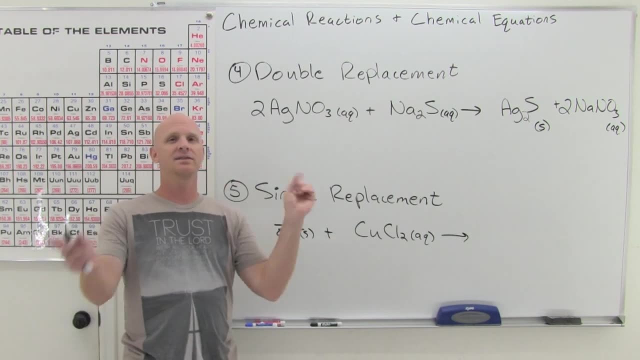 But we will cover them in Chapter four, when we revisit single replacement reactions again as well. But for now we just want you to be able to predict products and in a single replacement reaction, instead of having cations and anions trading partners, you're going to have whoever's starting. 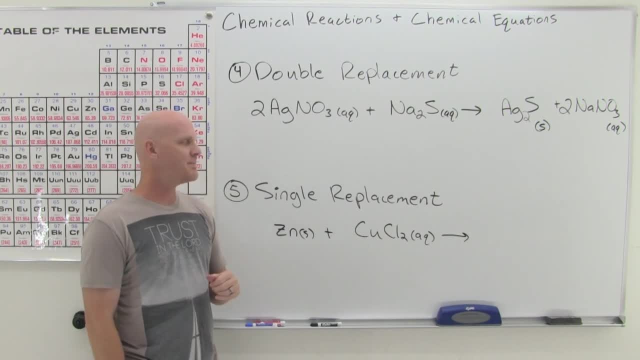 off alone, replacing somebody in another one, And so in this case, I like to think of copper and chloride. They're hanging out, They're together, They're a couple, and zinc's all alone, and zinc's like, hmm, I could be a cation instead of you, copper, and I could be with chlorine. 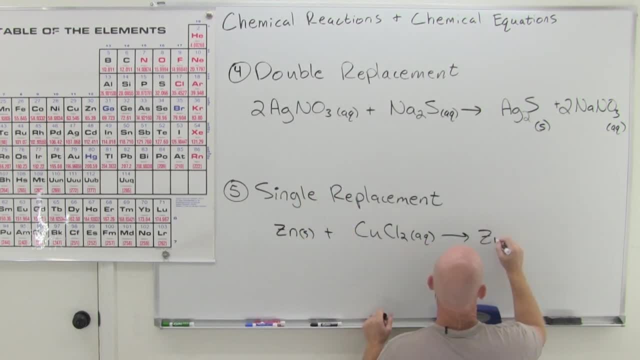 And that's exactly what we're going to write here. So we're going to have zinc combining with chlorine and that's going to leave copper all alone, And in this case again, if you recall, cadmium and zinc were ions that you're supposed to arise, that always are plus two as ions. 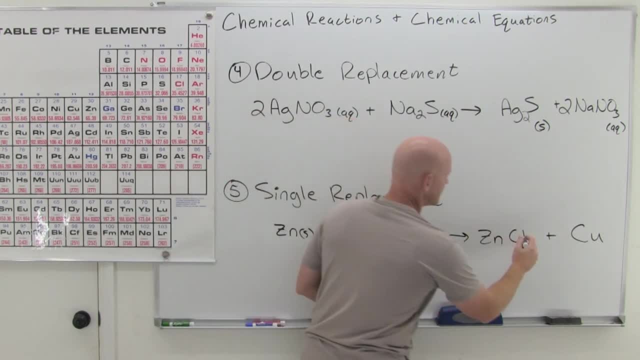 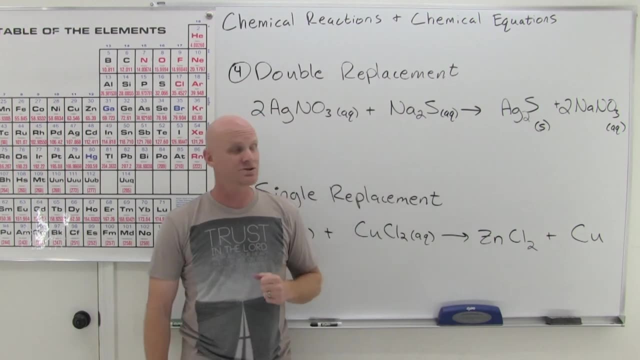 And so zinc is plus two and chlorine is plus one. Well then, I'm going to need another chlorine to make that balanced out as well. And again, don't just see: well, there's two here, So there's got to be two here. That's not always true. 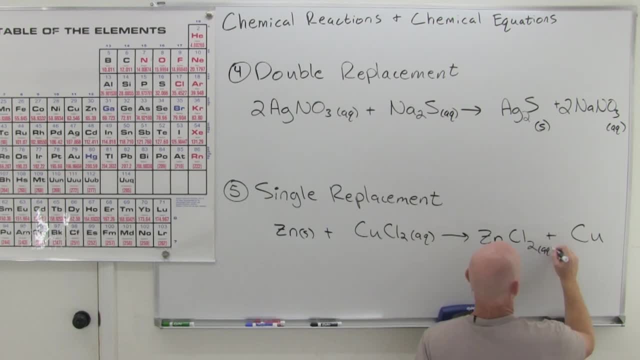 Cool. And it turns out that the zinc chloride here would be aqueous. but the copper is now all alone. And when zinc's all alone, zinc metal. when copper's all alone, that's copper metal, and copper metal is a solid at room temp. 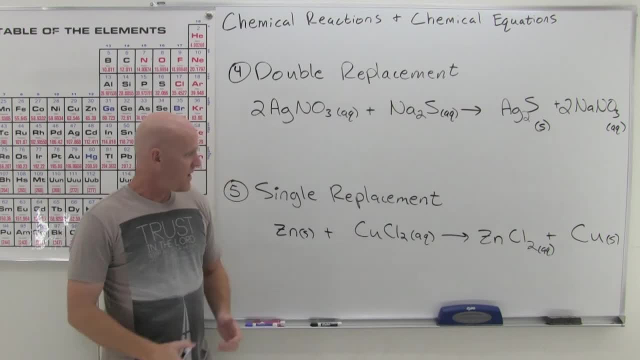 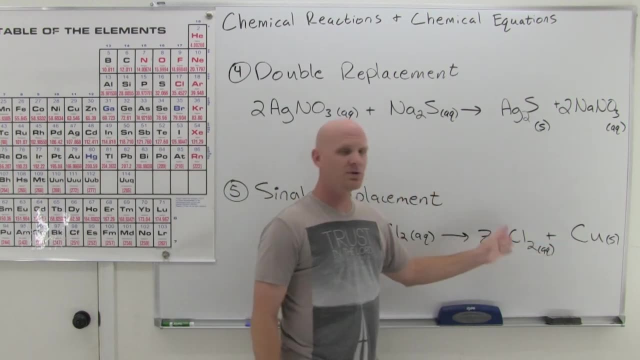 So we'd put a solid there And in this case we go to balance this and we'll find out that actually it is already balanced. We have one zinc and one zinc. We have one copper, one copper. Two chlorines, two chlorines. 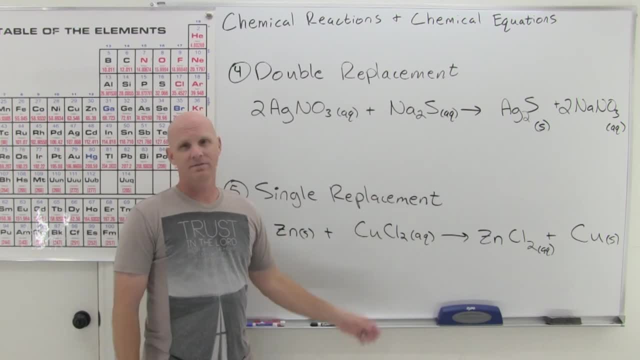 And this one was not so bad. These can get a little bit complicated and stuff like this. We get to bigger redox, but for single replacement they usually end up being pretty simplistic to balance, just like this. Cool, And that is all. five types of reactions. 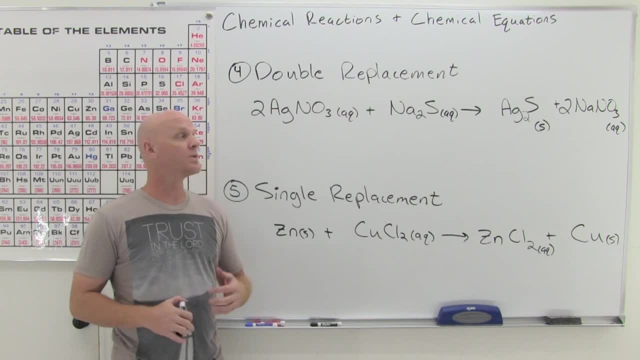 And again, we're not going into crazy detail just yet, but it turns out we're going to reference some of these in the later lessons here in Chapter three. So that's why they- one of the big reasons they had to get brought up now- 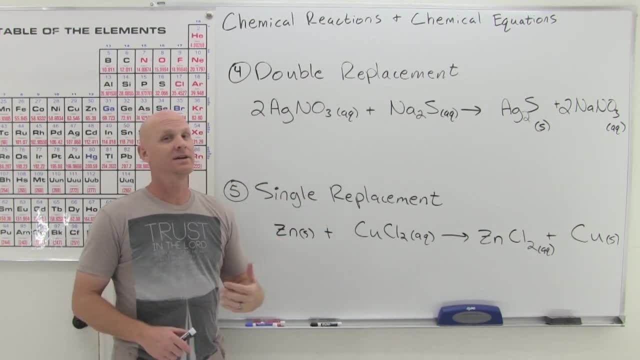 But, like I said, these last two, we're going to discuss them again In greater detail in Chapter four. Now, if you found this helpful, would you consider giving me a like and a share? Best thing you can do to make sure YouTube shows this lesson with other students as well.